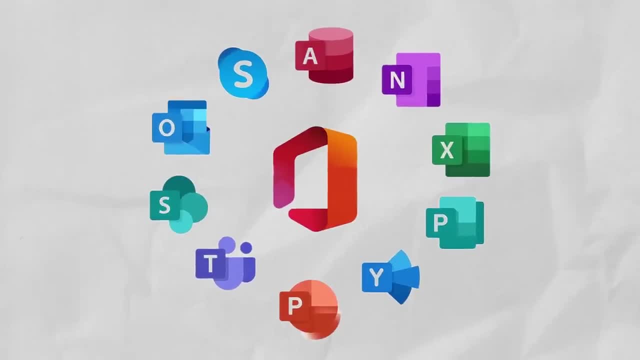 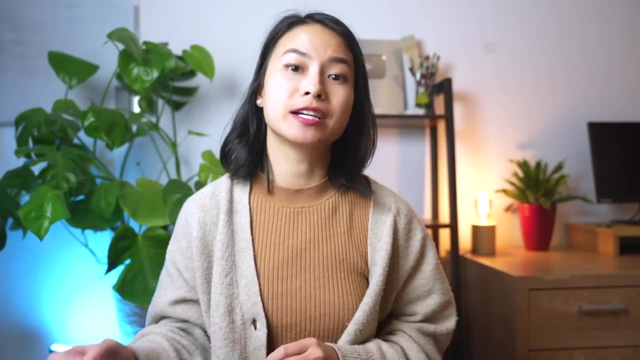 launched very soon, which brings AI to all Microsoft Office applications. So if your hands touch keyboard for work, this is going to change your job in the next few years. This motivates me. If there's something that's gonna change my life and work forever. 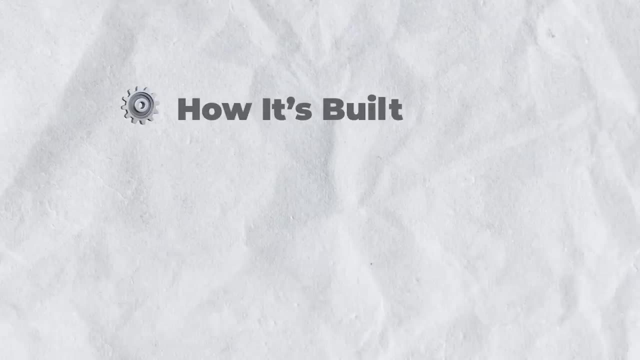 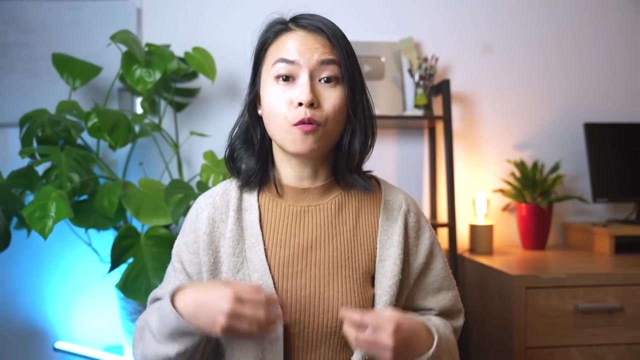 I want to learn everything about it. I want to learn how AI is built, how to build with AI and how to use it to enhance my work. I think, as someone working in the tech field, you want to be in the position where 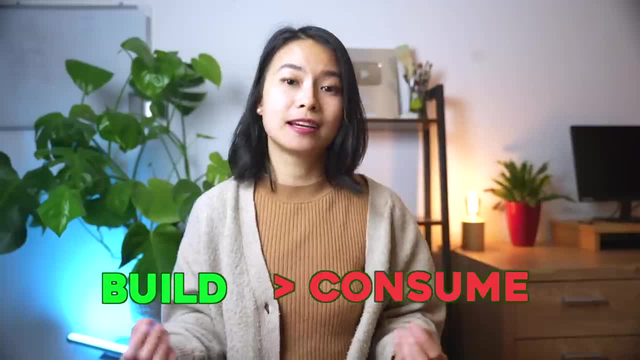 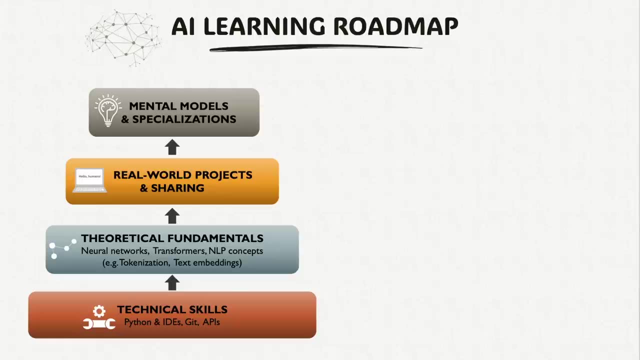 you can build things with AI rather than just consume it. So today I'll be sharing with you a roadmap as a one-stop shop for you to expand your AI skillset, Learn the fundamentals of AI and learn to build with AI, Even if it's just a simple tutorial. don't forget to subscribe to my channel and turn on the bell. 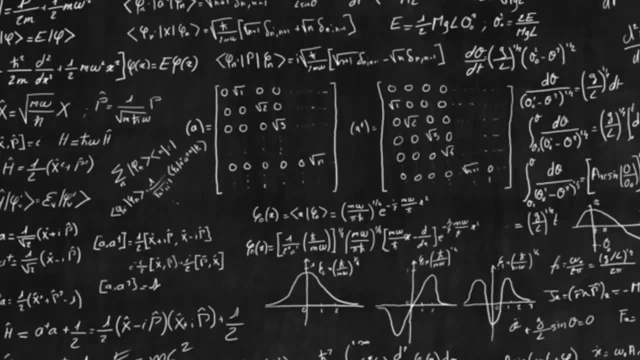 you'll get to know the next video as I upload more videos every Friday, So don't forget to share this with you and share this with your friends over time If you're not already subscribed to my channel. you don't have any background in machine learning, mathematics, statistics or programming. I hope. 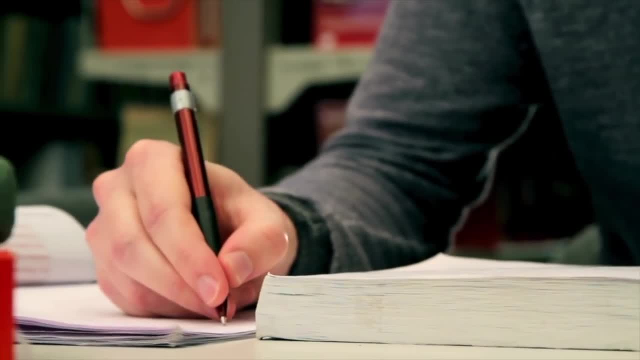 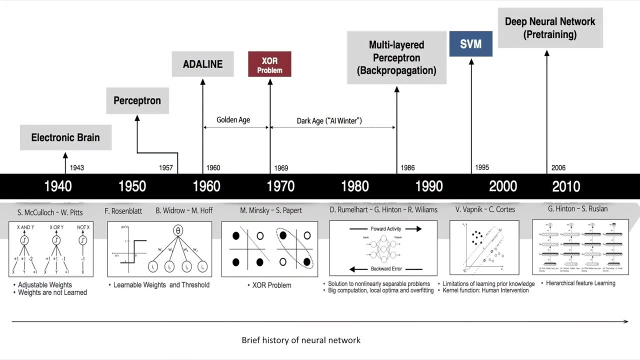 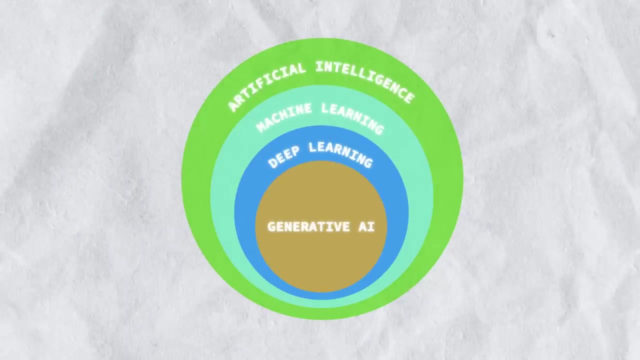 you'll walk away with some useful ideas of where to start. Let's get started. So why should we bother learning AI? This whole AI, machine learning and deep learning thing has been around since the 1950s. The AI we often talk about today is generative AI, which is a subset of machine. 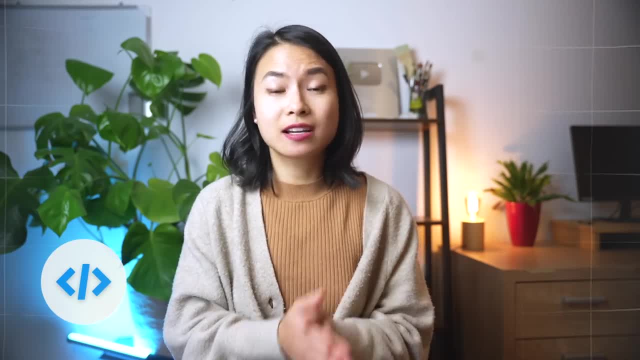 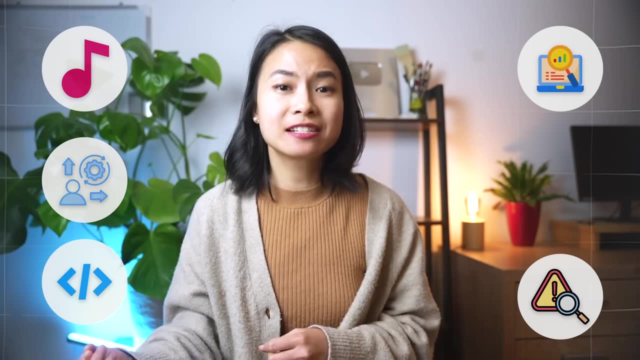 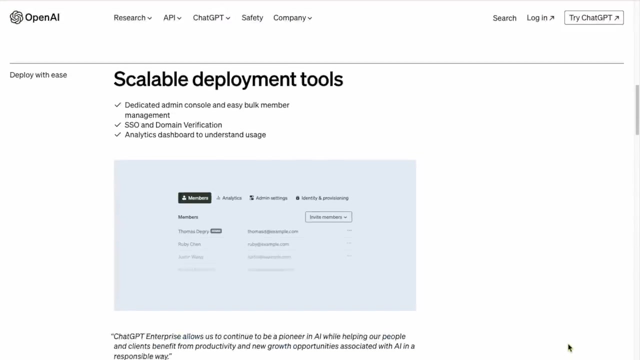 learning and deep learning. Generative AI can now write code, generate stunning images, writing music, diagnosing rare conditions, creating outline for presentations, reading images and much, much more. Companies are looking into implementing AI solutions to solve their specific problems. This. 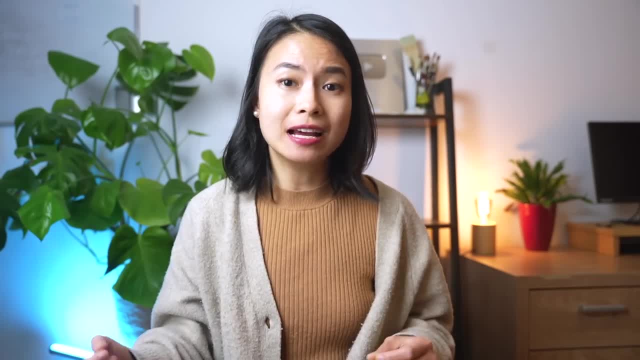 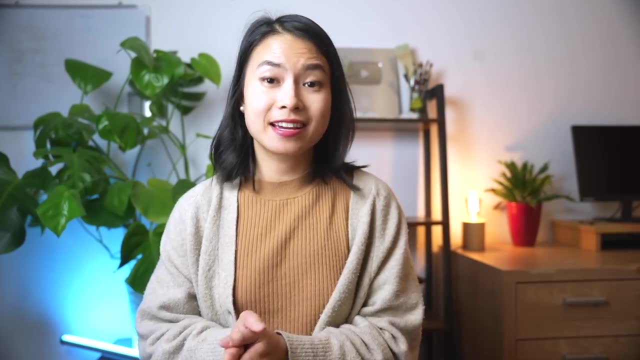 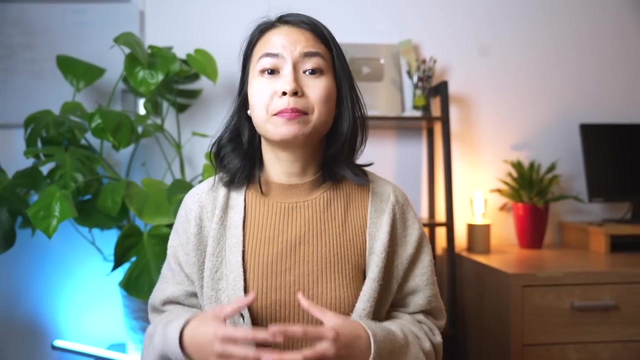 is a goldmine because everything is still so new. So if you have the knowledge and know how to build things with AI, you can create huge impact. As with anything in its early days, you can still have many issues that need to be solved. They are not yet reliable or stable. They 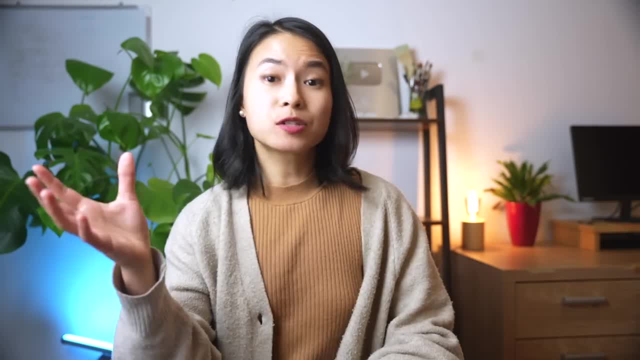 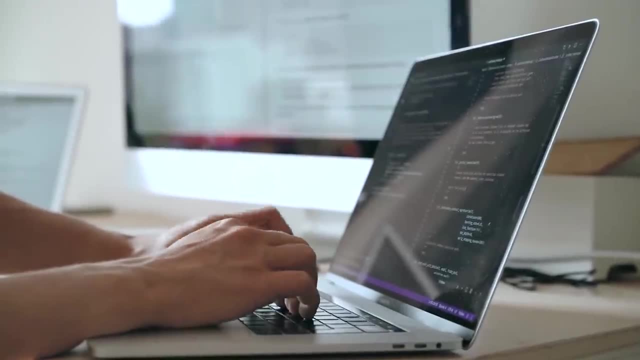 potentially possess biases, among other things. That's why we need more people who have the in-depth understanding and can get to the bottom of the technologies to solve various problems. Even if you don't build things yourself, the knowledge can help you avoid a lot of misunderstanding. 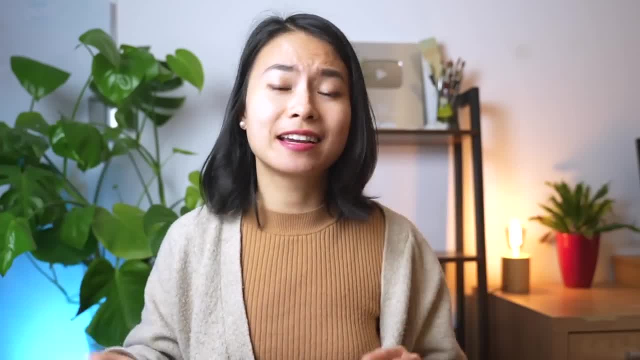 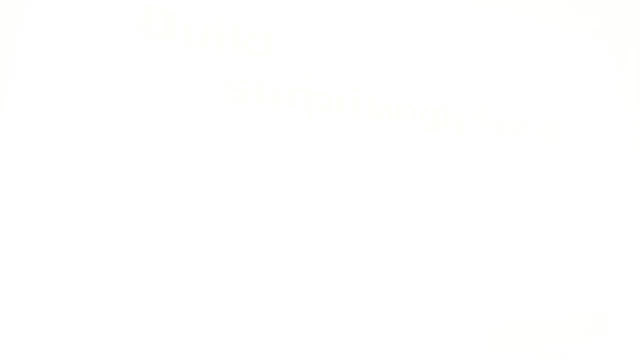 and misinformation, such as. AI can do everything, as long as you got the right plugins. Okay, when it comes to learning AI, we're going to talk about how to build a machine learning AI, So let's get into it. Of course, there's no one-size-fits-all roadmap. You might have seen a lot of low-code or no-code. 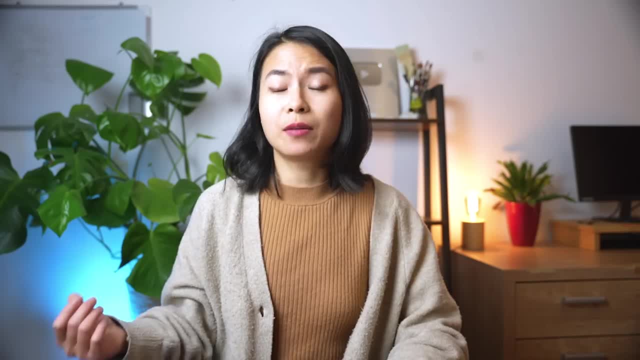 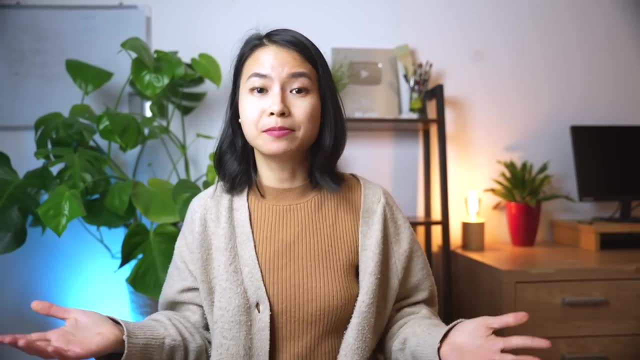 tools to help you get started with AI and even develop things like an AI chatbot. You can certainly play with them to have the first feeling of how things work and what is possible, and even build great real-world solutions with them. As you get more into it, you might realize that those 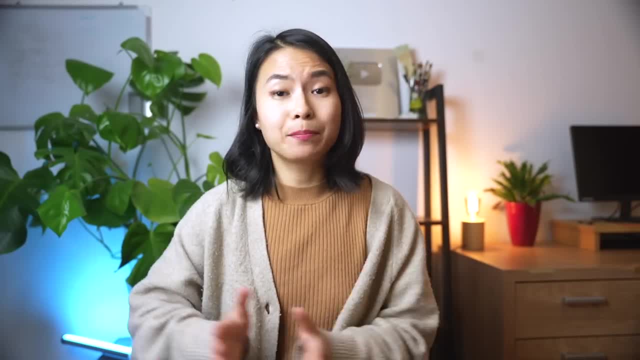 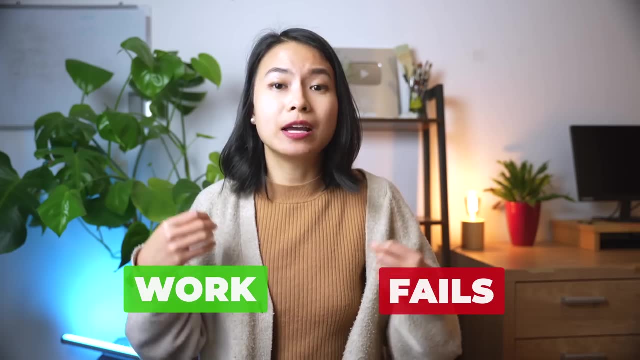 tools might feel like a little bit of a black box. They might not be so flexible that you can customize a lot of things, or sometimes they're not so flexible that you can customize a lot of things. Sometimes your solution works and sometimes it fails. So if you really want to, 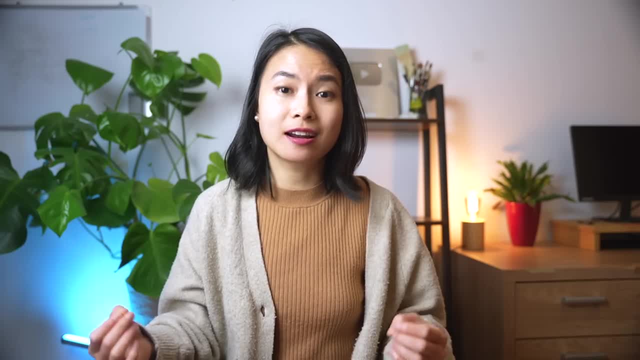 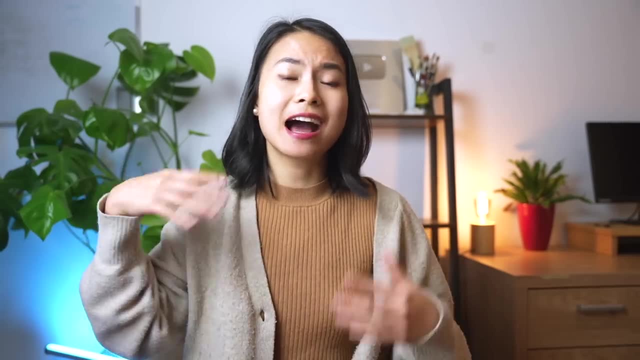 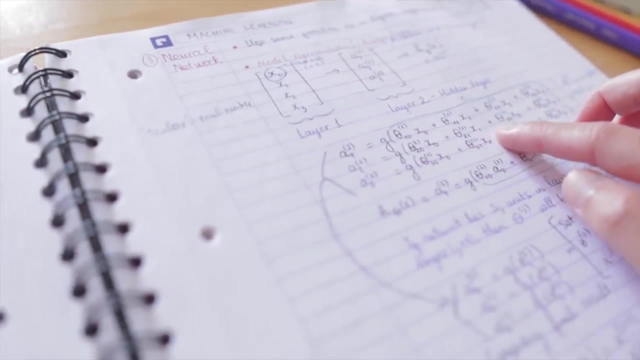 learn how artificial intelligence works and build tools that are reliable, scalable and can be tailored to your specific use case. I think that's when you hit the ceiling and can't rely solely on those low-code platforms anymore. Personally, I often prefer to have a solid understanding of 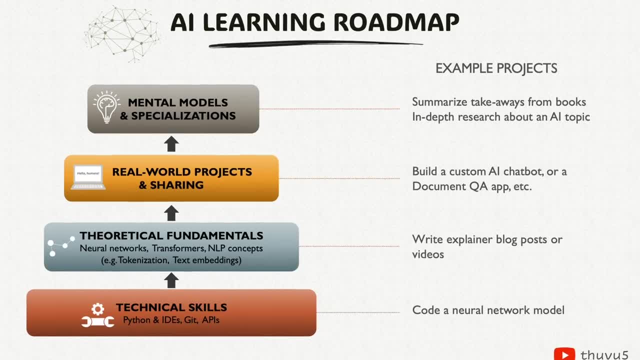 how things work from ground up, So let me walk you through a roadmap for learning AI. You can download this full roadmap in PDF, together with my link in the description below, And if you want to learn how artificial intelligence works and build tools that are reliable, scalable and can be. 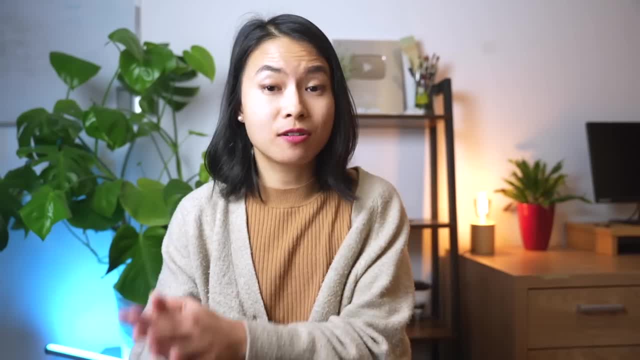 tailored to your specific use case. I think that's when you hit the ceiling and can't rely solely on those low-code platforms anymore. So let me walk you through a roadmap for learning AI. You can find the link in the description below. On the fundamental level, you want to learn the basics. 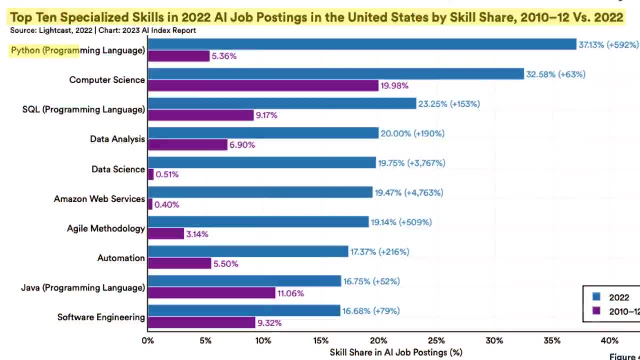 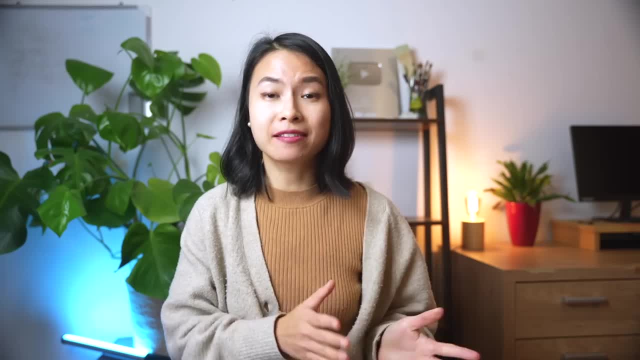 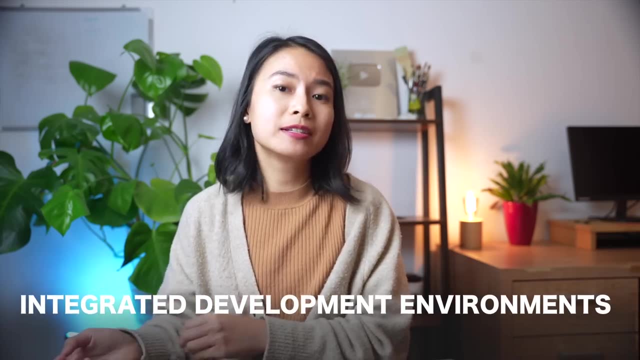 of programming. Python is one of, if not the most, used programming languages for machine learning, deep learning and AI, So some coding knowledge in Python would be essential. For working with Python, you can certainly use several IDEs or integrated development environments, For example. 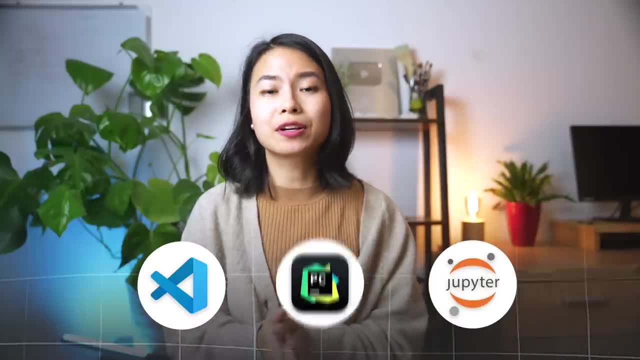 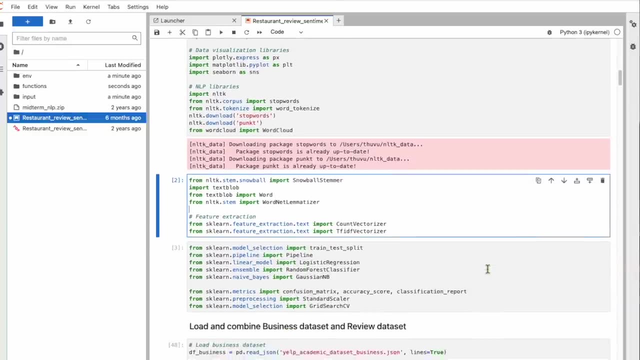 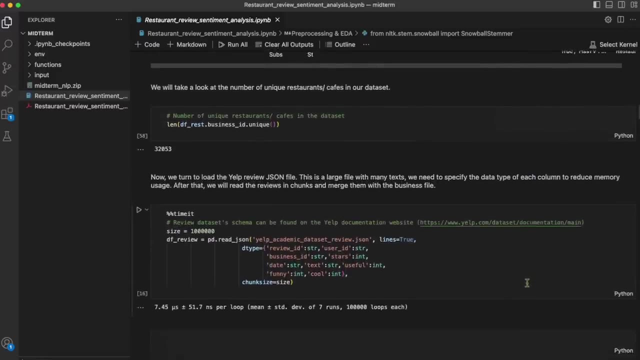 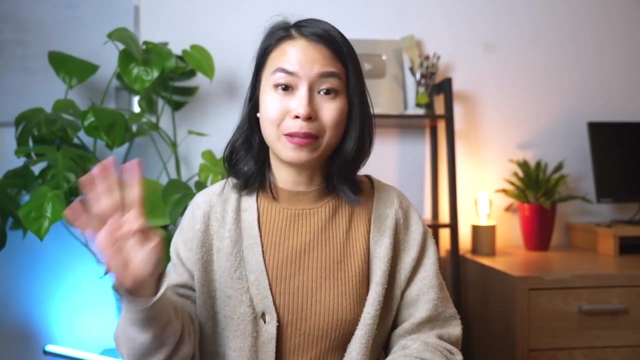 Visual Studio Code, PyCharm or Jupyter Notebook. Jupyter Notebook is a software that allows you to use any of these tools, and they are completely free. If you've never coded in Python before, make sure to at least get yourself familiar with the four basics of Python. Firstly, data types and 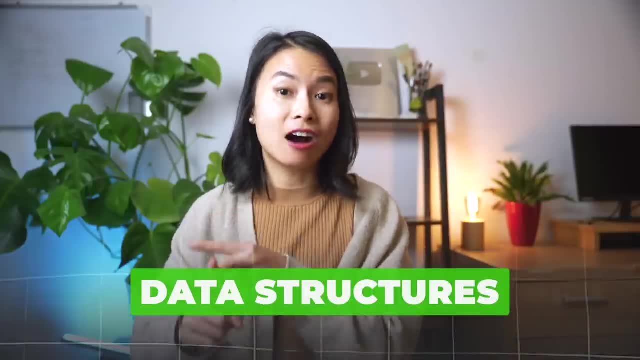 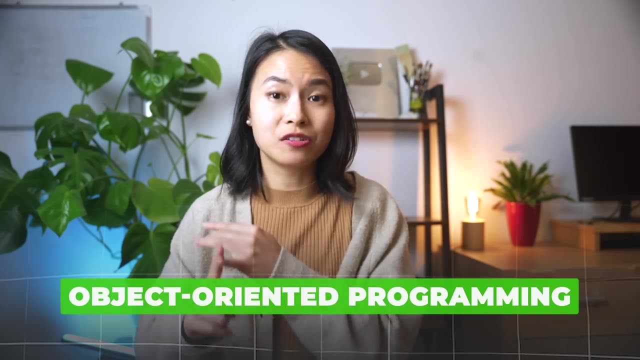 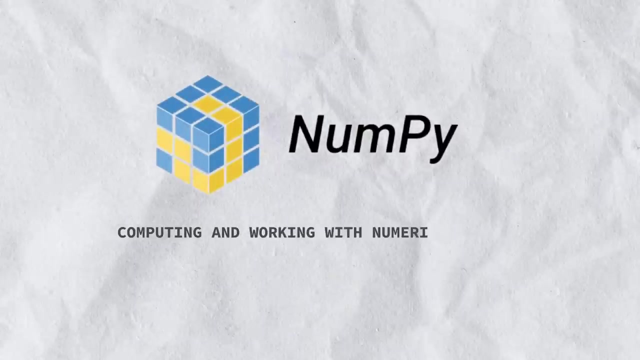 the operations that you can do on them. data structures and how to work with them. conditionals, loops and functions. And lastly, project-oriented programming and using external libraries. When learning Python, the most essential libraries to learn are NumPy for computing and working with numerical data. 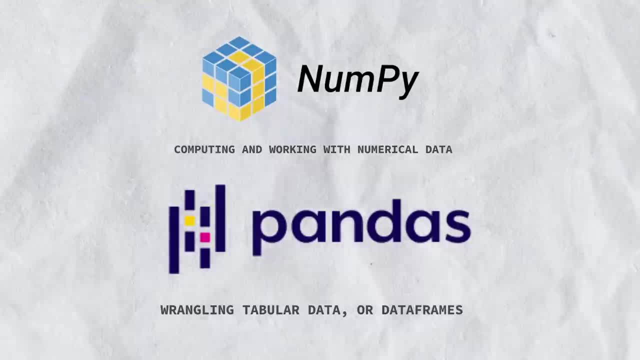 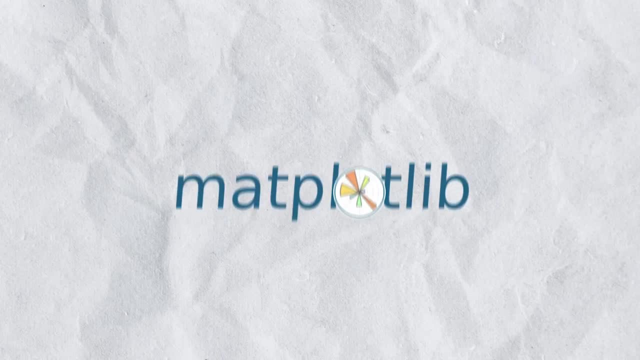 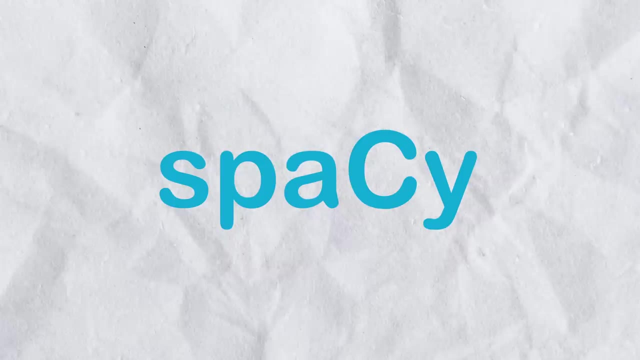 Pandas for wrangling tabular data or data frames. When you're already familiar with those libraries, you can start learning some other libraries that you can use for your AI project. For example, Matplotlib is a popular library for data visualization, spaCy for basic text processing. functionalities and so on. For example, Matplotlib is a popular library for data visualization, spaCy for basic text processing functionalities, and so on. For example, Matplotlib is a popular library for data visualization, spaCy for basic text processing functionalities, and so on. For 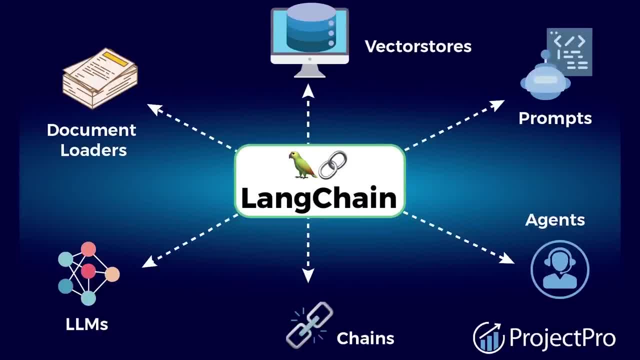 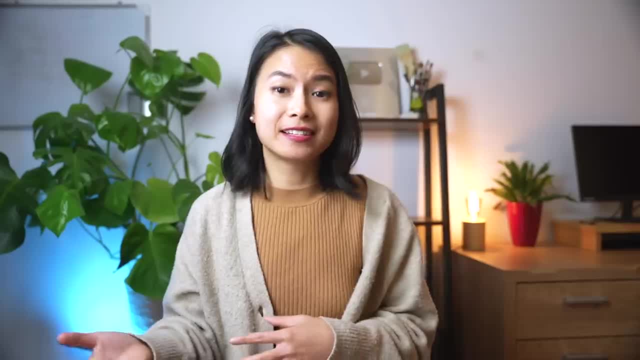 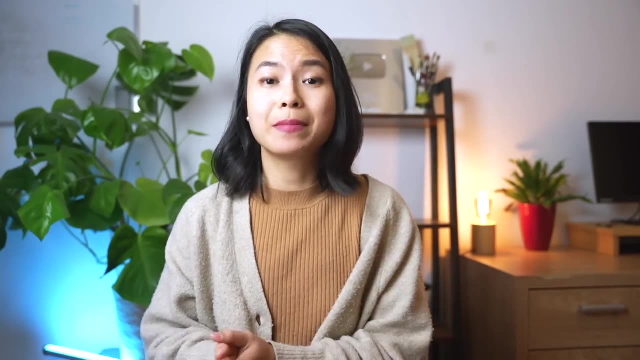 working with large language models. LangChain is a very useful library to learn to develop multiple applications on top of LLMs. What's nice with Python is that there are so many open source libraries that you can use to develop almost anything you want. The next thing I'd recommend: 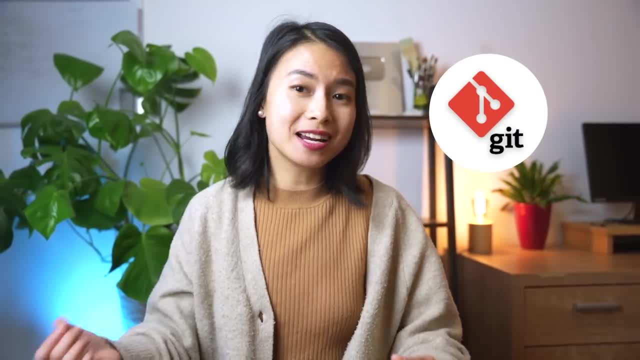 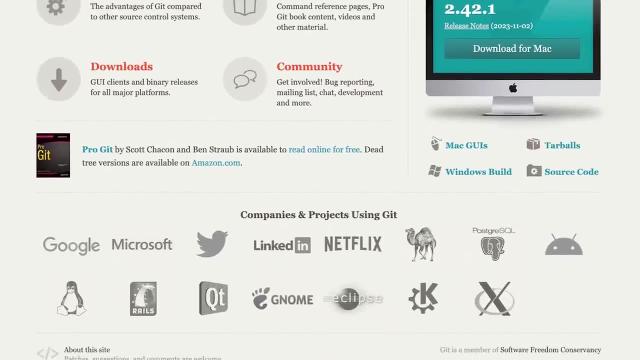 you learning is Git version control. If you're not yet familiar with it, Git is an open source software for tracking changes in your project, basically managing versions of your project. Git version control is an open source software for tracking changes in your project, basically managing versions of your project. 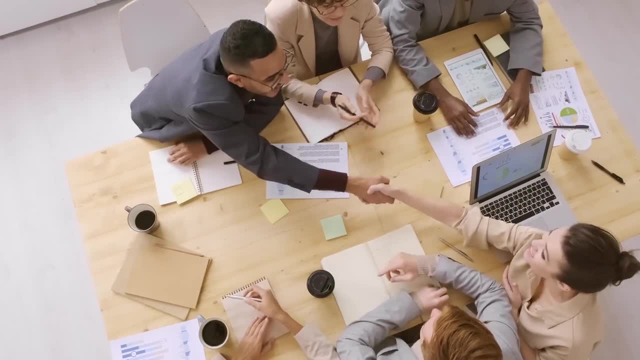 Git version control is an open source software for tracking changes in your project, basically managing versions of your project. Git version control is an open source software for tracking changes in your project, basically managing versions of your project When you're collaborating with other people in a large or complex project. there are actually just 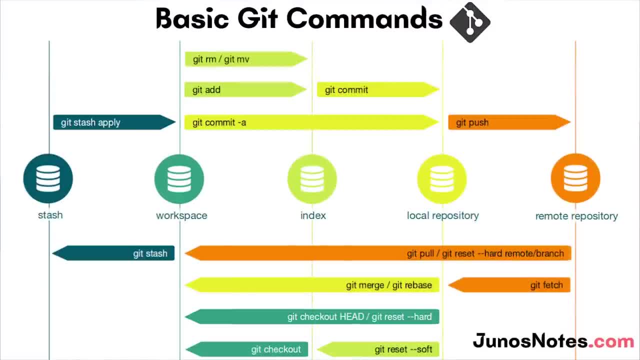 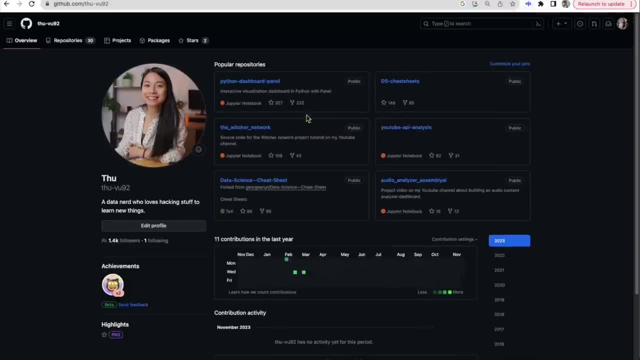 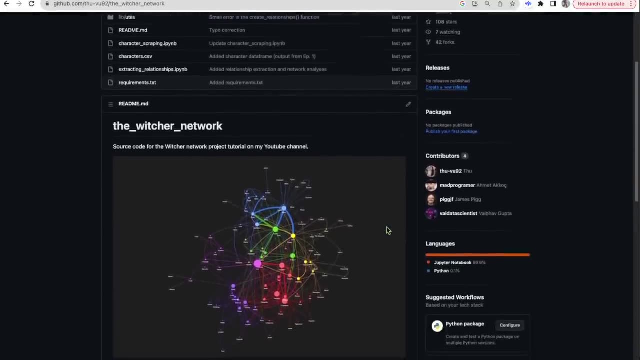 a few concepts you need to understand to start using Git, as shown in this diagram. A funny thing is that many people actually confuse Git with GitHub. GitHub is a hosting platform for Git repositories so that you can share your project with other people across the internet. 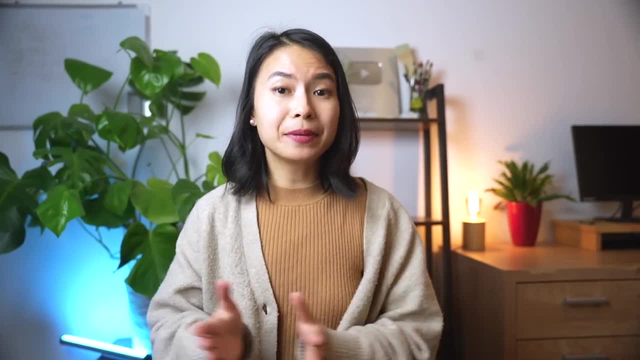 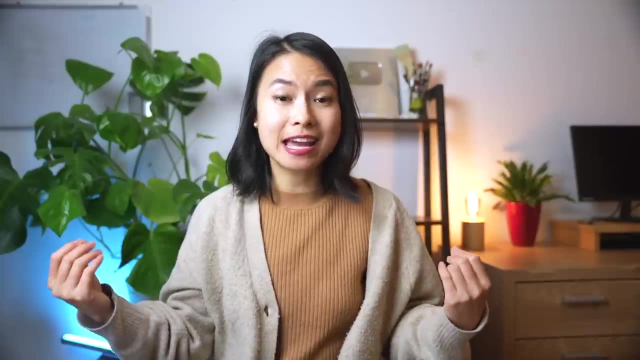 Meanwhile, Git is the software itself. Through GitHub, you can directly see and contribute to other people's projects. So how can you start using Git? The easiest way is to install GitHub Desktop. It's a user interface tool to help you work with Git. 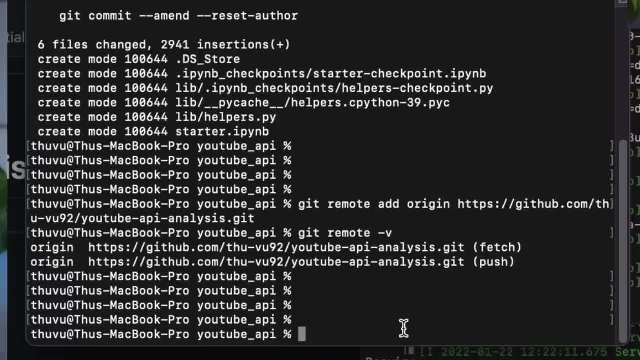 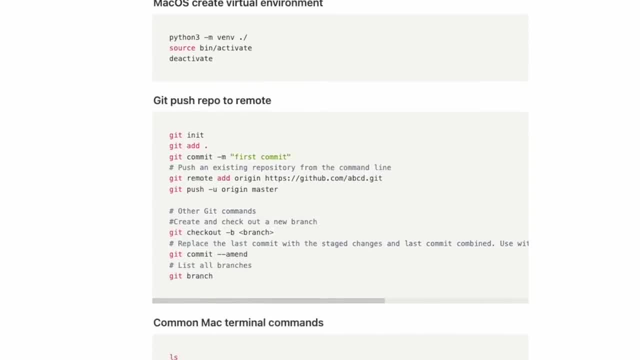 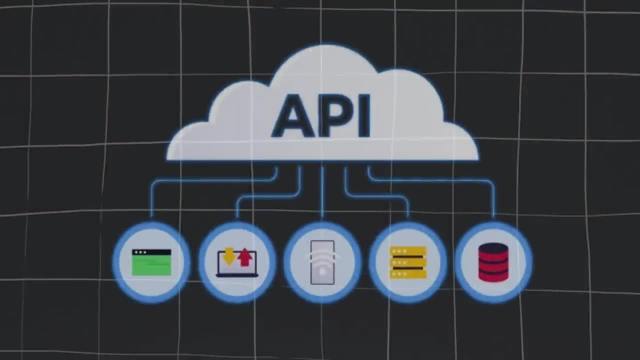 Or, if you prefer to use the terminal, you can also interact with Git through the terminal comments. I always keep a small cheat sheet here to remind me of some common Git comments which I find super convenient and helpful. Another essential thing to learn in your AI journey is using APIs, Knowing how. 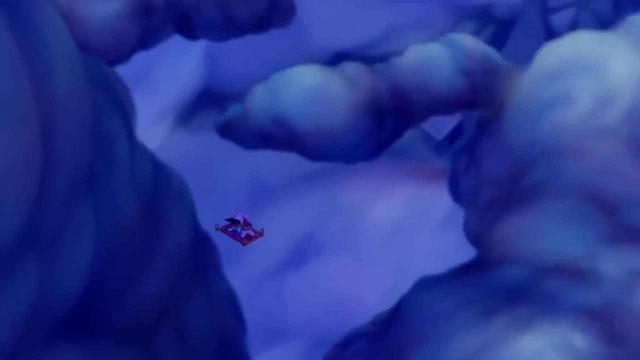 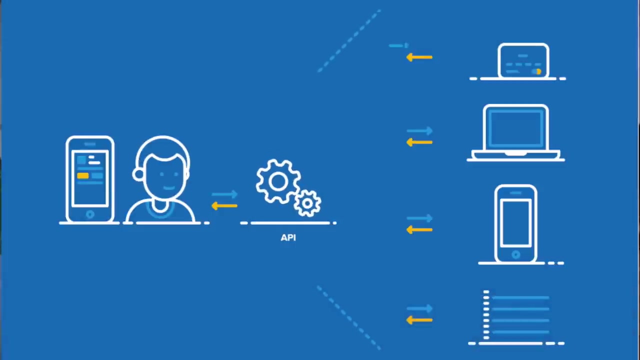 to use APIs is a magical skill that opens up a whole new world of possibilities. API stands for Application Programming Interface. It's a way for computer programs to communicate with each other. Basically, there are two jargons you need to learn. Yeah, just two. 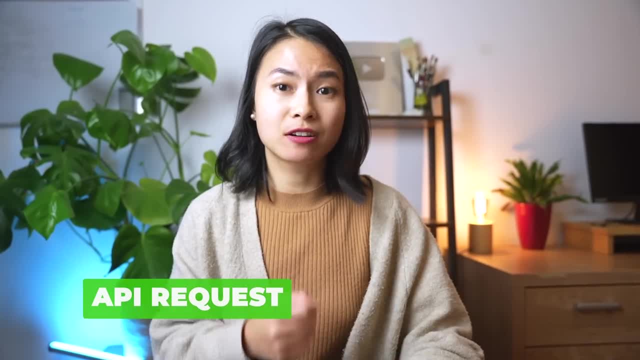 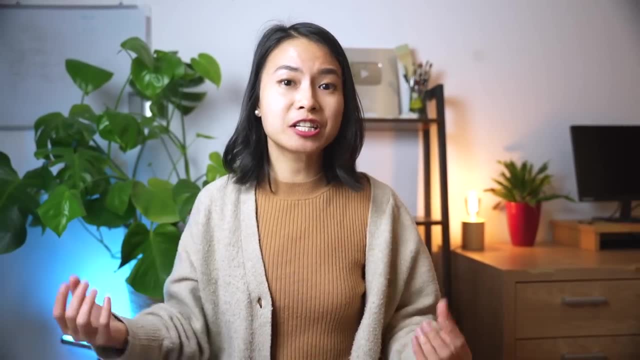 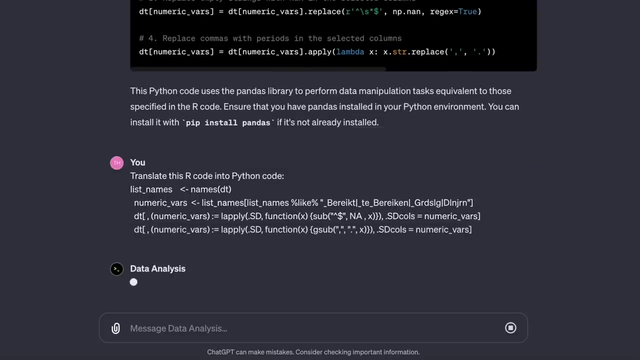 API request, which is also referred to as API call and API response. Depending on the API, you can make a request for data or for model prediction. in the case of ChatTPT, without knowing how to use the API, you'll be limited to the chat interface on the OpenAI website. Don't get me wrong. 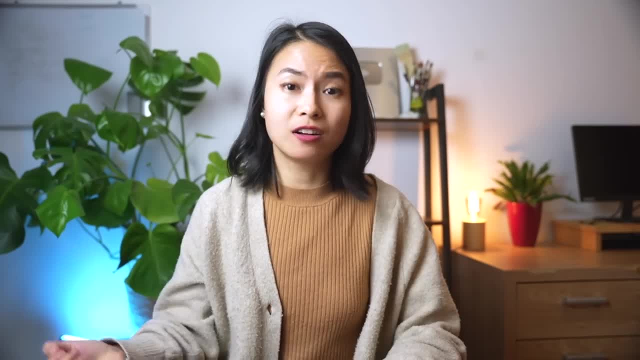 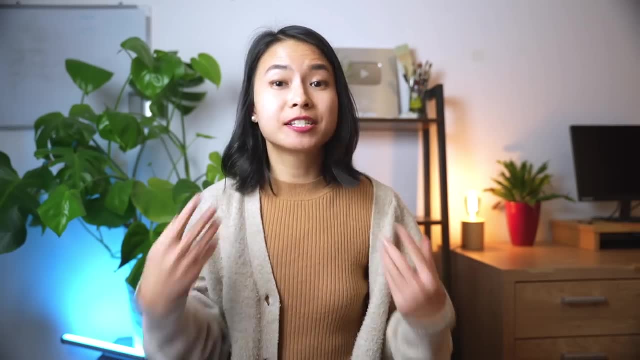 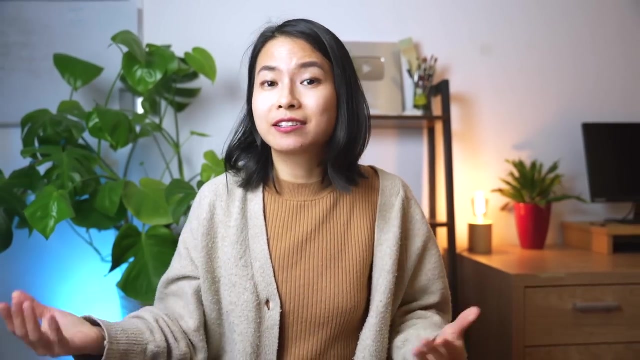 I love the ChatTPT website, but you can't develop your own tool this way or integrate the AI model into your current system. Okay, on to the next level. We're concerned with the theoretical fundamentals of AI. I recommend you at least get some high-level theoretical understanding of AI. 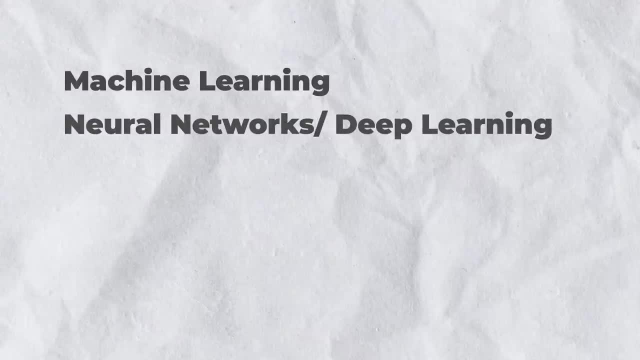 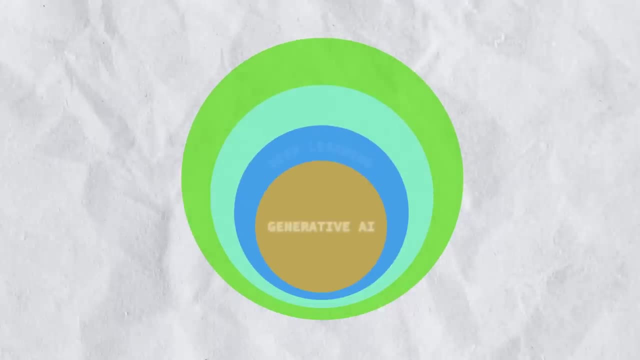 and its subfields, such as machine learning, neural networks and deep learning, and optional computer vision, NLP and reinforcement learning. Okay, if we look at this diagram again, deep learning is a subset of machine learning, Traditional machine learning algorithms mostly. 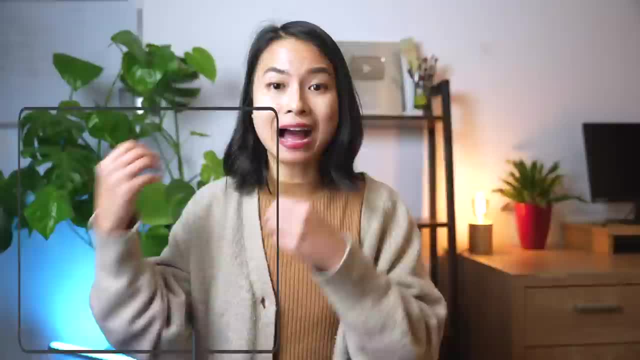 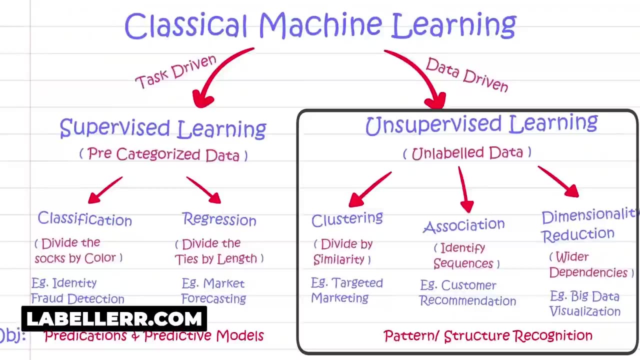 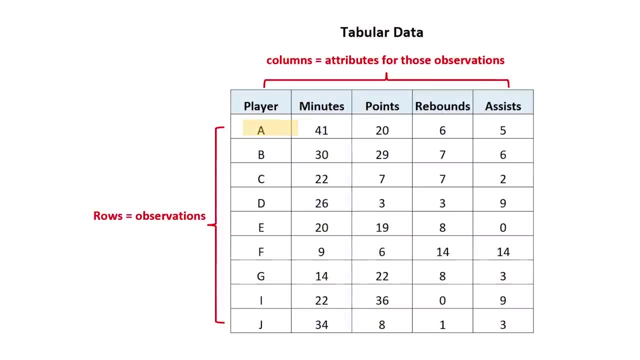 fall into either supervised learning- this is when you actually have the target labels to train the prediction model on- or unsupervised learning, when there's no target labels. In general, these algorithms only work for tabular data. Think of data tables with each record being a row and 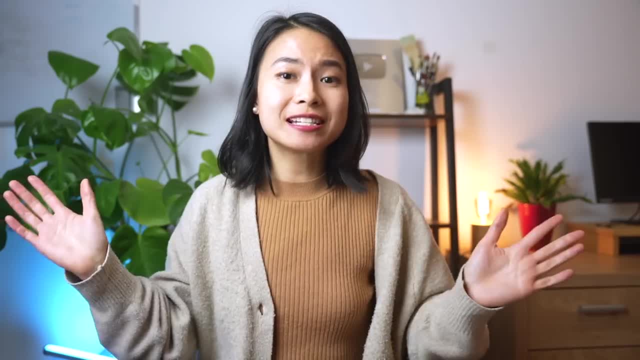 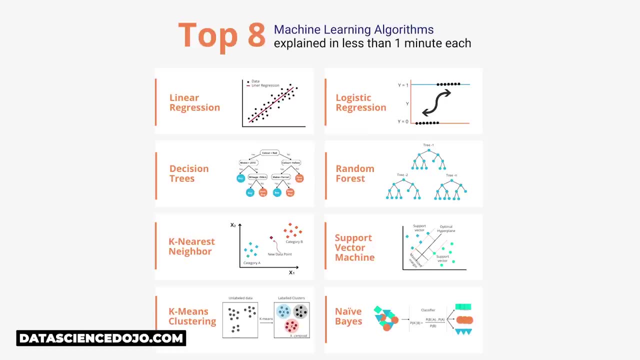 data feature being a column in that table. If you're interested, you can quickly go over some machine learning jargons and get some high-level understanding of these algorithms. They're all cool to learn, but since AI today uses deep learning, I think to save time, you can probably 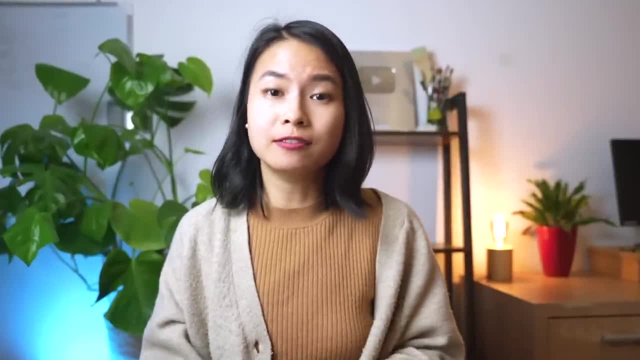 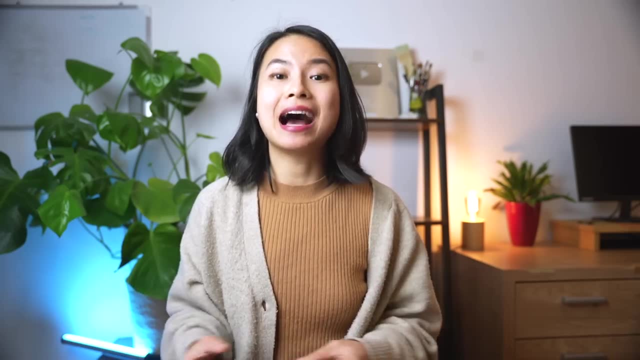 just jump right into deep learning. I think you'll anyway learn the essential machine learning concepts along the way. As we just briefly talked about, neural network is the algorithm behind deep learning. It works incredibly well for deep learning and it's also the most efficient way to. 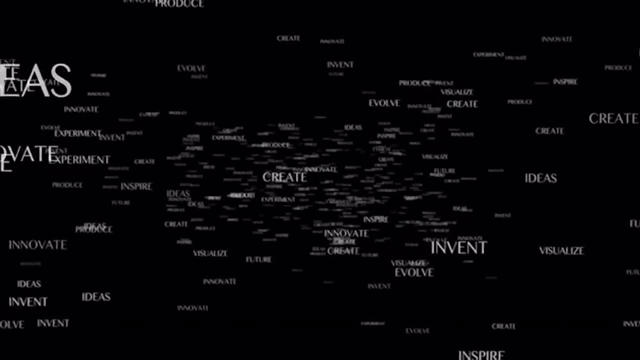 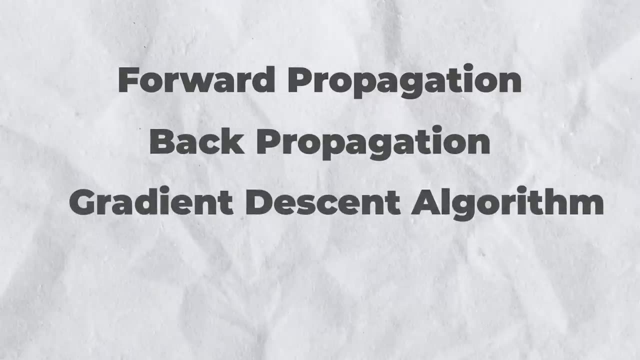 do so For unstructured data like text and images for a neural network. you want to understand the main concepts such as forward propagation, back propagation, gradient, descent algorithm and how weights are updated in the network. If you like some math, you can try to understand. 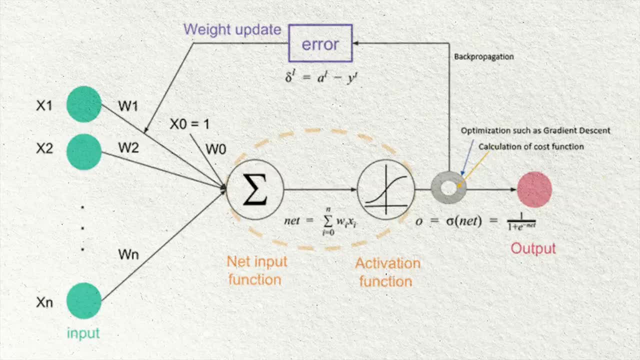 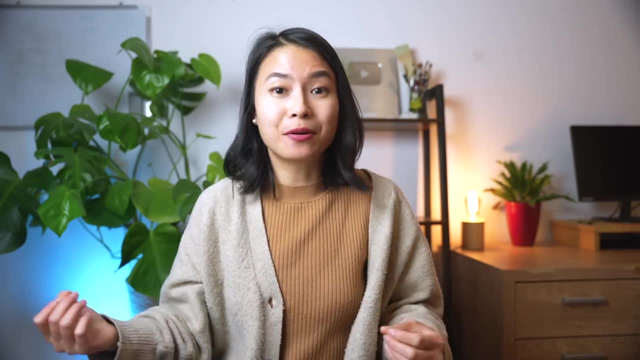 all the calculations underlying the neural network. They're really not too difficult to understand, so don't shy away from it. Neural network in itself is pretty simple and maybe even a bit inferior to deep learning, but it's still a great tool for deep learning, If you're. 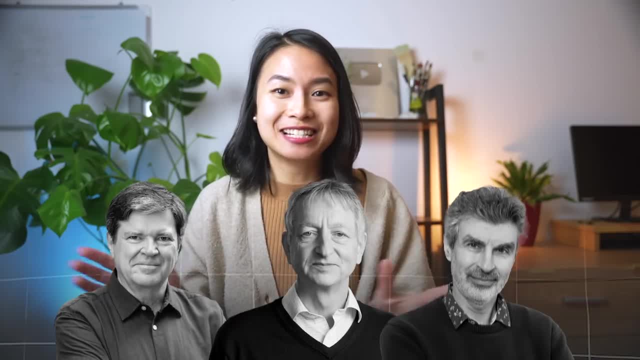 interested in learning more about deep learning, please subscribe to my channel and I'll see you in the next video. Thank you for watching and I'll see you in the next video. No offense here to the fathers of deep learning, but when you stack many, many network layers, 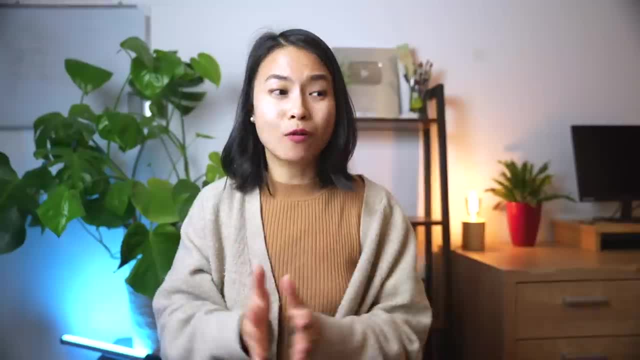 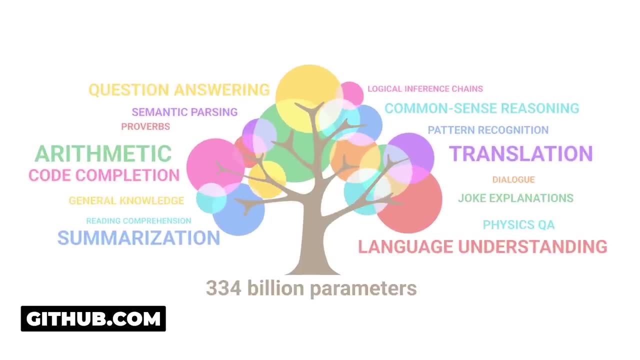 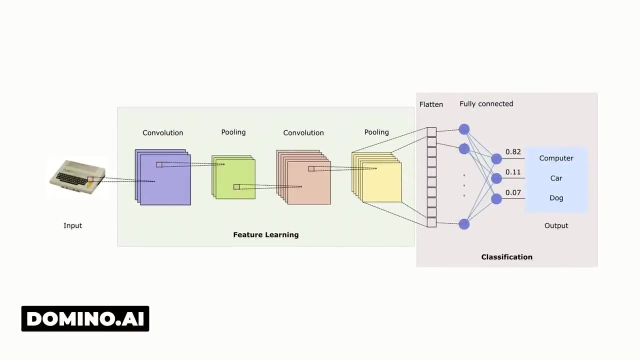 together into a complex architecture. this is when things get interesting. The neural network now can start recognizing digits, classifying cats and dogs to predicting the next tokens. in the case of LLMs today, Convolutional neural networks used to be a very popular architecture. 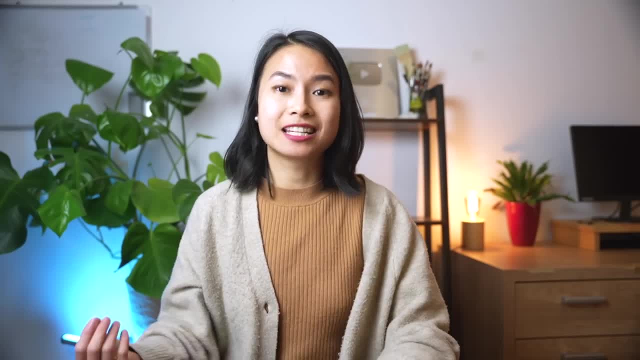 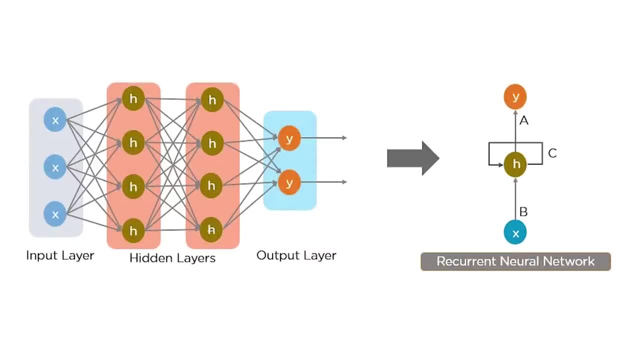 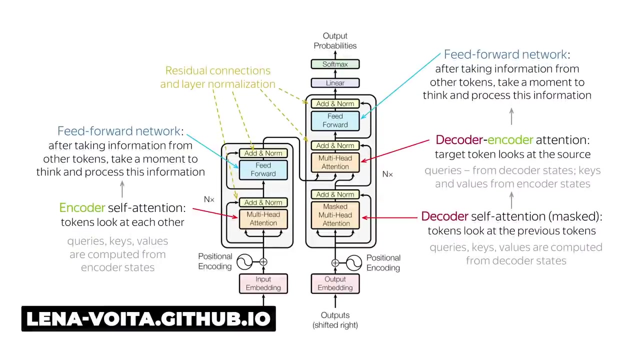 for deep learning with images because it can recognize patterns on images And recurrent neural networks used to be very popular for text modeling because it can understand sequences. However, these architectures have become pretty obsolete since the invention of transformers architecture in 2017.. This is the architecture behind the foundation language models. 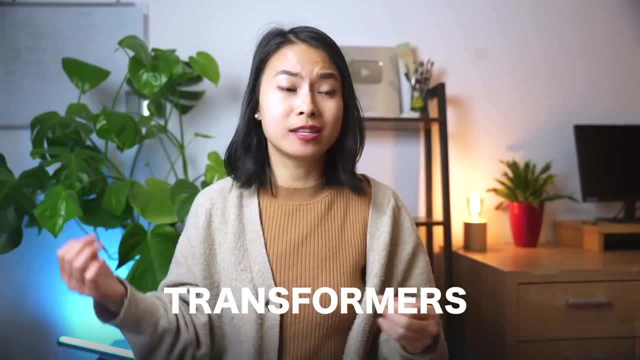 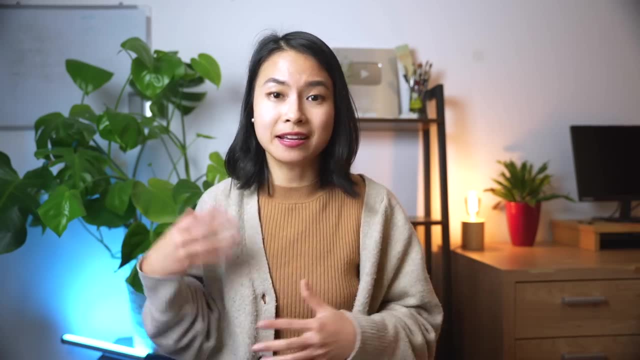 nowadays, Transformers outperform pretty much all the earlier architectures, so you might want to jump into it right away and reverse engineer the knowledge if you see any gap. As you work with the AI models, you also want to get yourself a high-level understanding of how the foundation 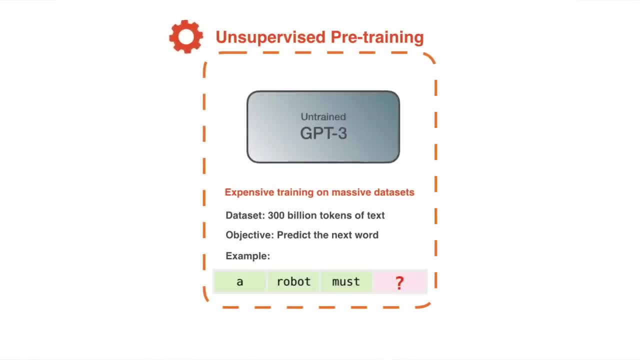 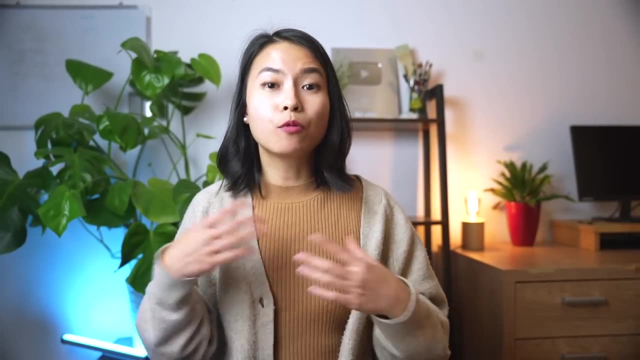 models underlying them are trained. In general, they're trained through an unsupervised process. It's up to you to learn more about the nitty-gritty details of training your language models. When working with language models, you might hear the common term 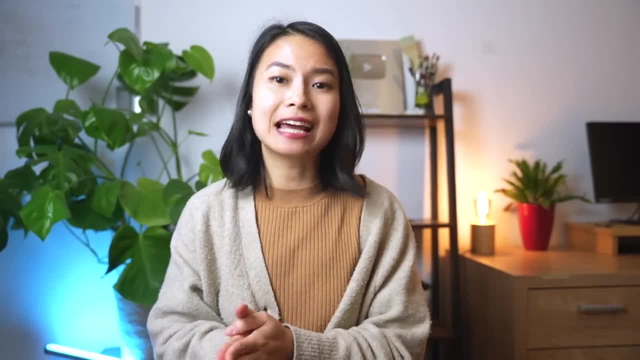 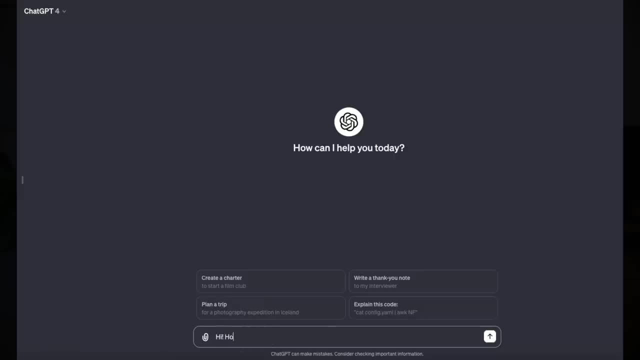 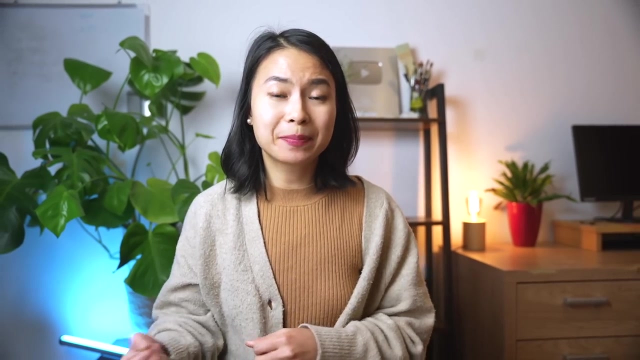 text embeddings. This is a very useful concept to understand. Text embedding converts text into vectors of numbers. Nowadays we often forget that computers- not only computers, but even computers- cannot actually understand human languages. Computers can only understand numbers, So this conversion step is really necessary. 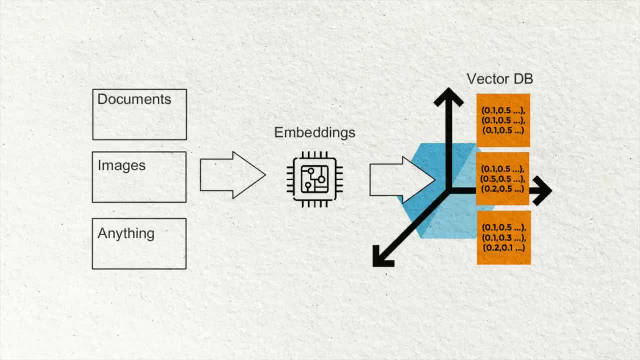 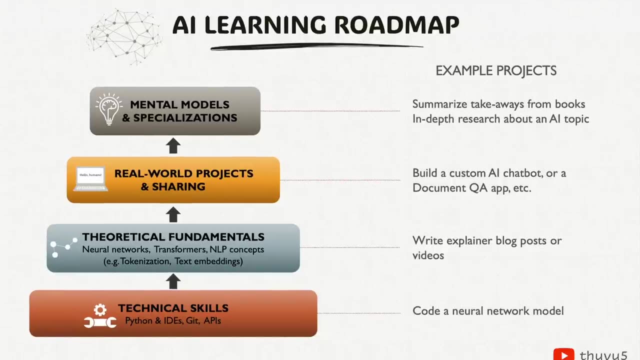 There have been many embedding models created with ever-smarter ways to capture meanings into those vectors. No matter what you're learning or where you are on this journey, you can build relevant projects to get your hands dirty and experiment with things. This will help you connect. 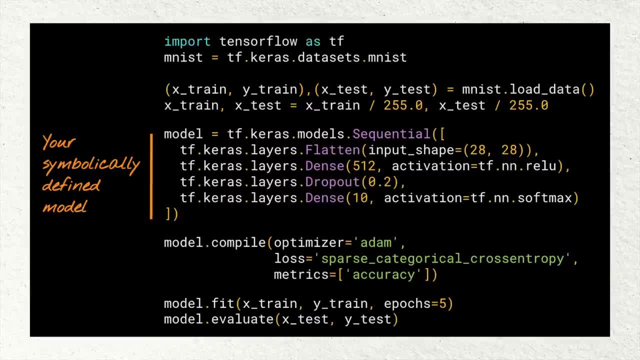 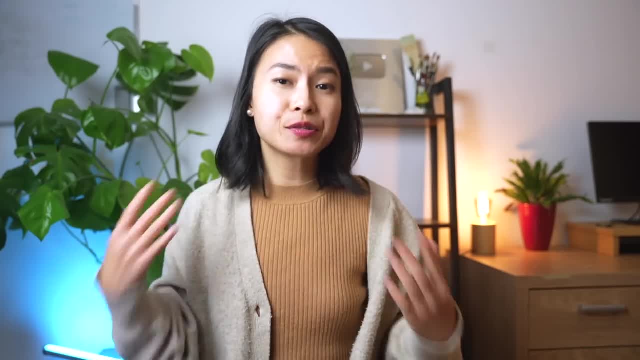 the dots and challenge your own understanding. For example, if you're learning Python, you can build your first neural network in Python using Keras or TensorFlow library. It's only a few lines of code. If it's too high-level, you can try to write a neural network and implement gradient descent. 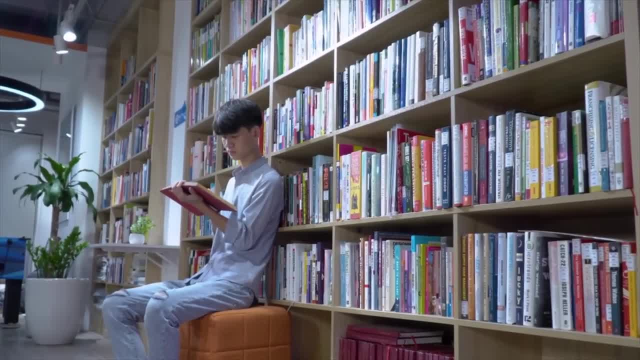 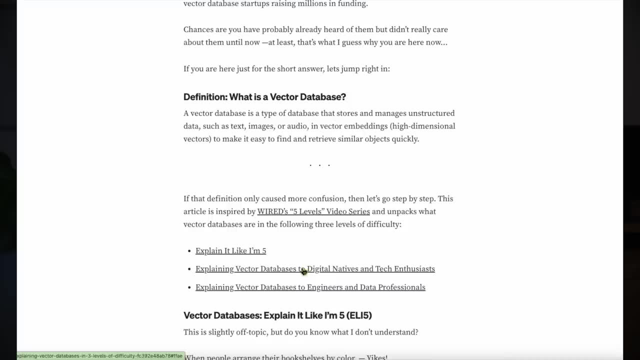 from scratch with NumPy When you're learning the theories. a real-world project would be to pick one specific concept you find interesting and write a blog post or make a video on it. This will help you understand the concept deeper and help other people too, If you're ready to tackle. more complex AI projects. you can build your first neural network in Python using Keras or TensorFlow library. It's only a few lines of code. If it's too high-level, you can try to write a neural network and implement gradient descent from scratch with NumPy. It's only a few lines of code You can build. 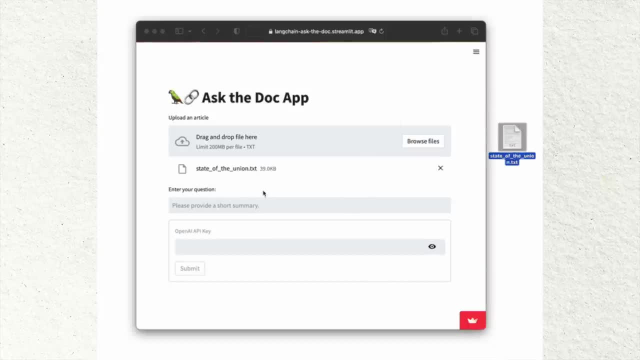 a real-world application. For example, you can create a document retrieval app, basically to create a chat with PDF kind of application where people can upload a document and ask specific questions based on the document, Or you can create your own chatbot. I also want to mention that no. 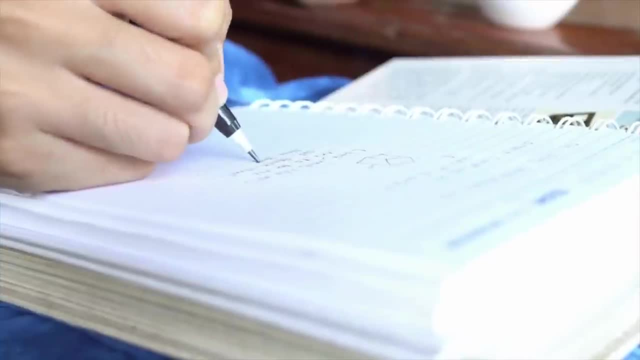 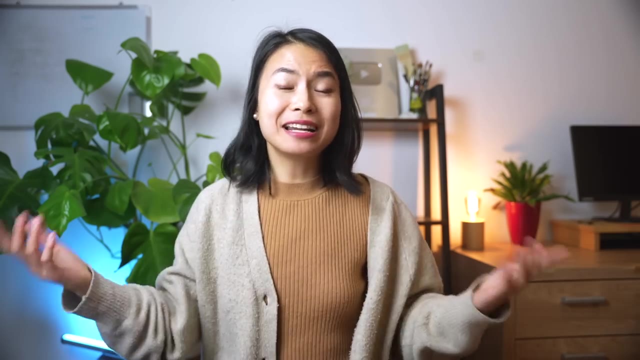 matter what project you do, big or small, make sure you document them for reference for yourself and share that with other people through articles and social media posts. You really never know how many people might find it useful. The next thing I'd recommend is to develop mental models around. 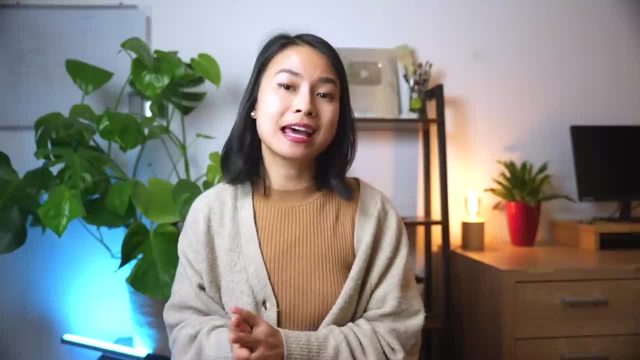 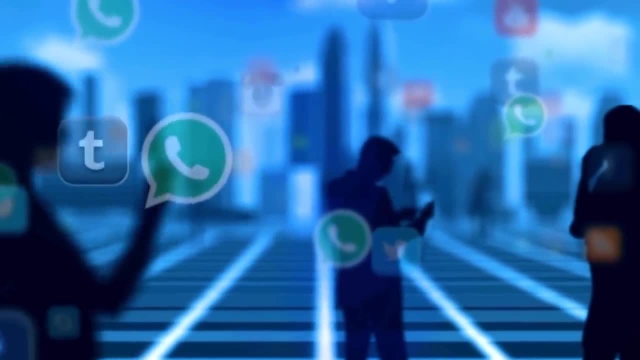 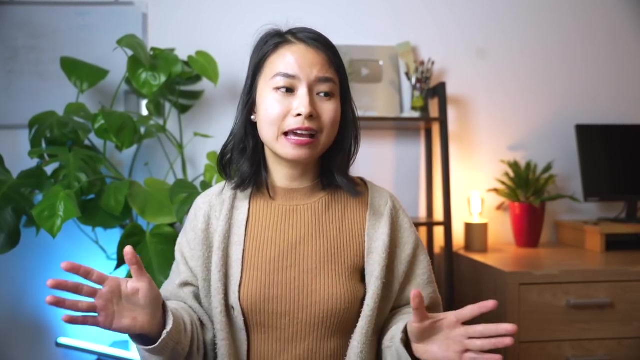 AI and perhaps specialize in a certain area within AI if you want to. I think reading books about AI is a great way to go through the noise on social media and get a more well-rounded background of AI. This also equips you with the right frameworks and tools to reason and 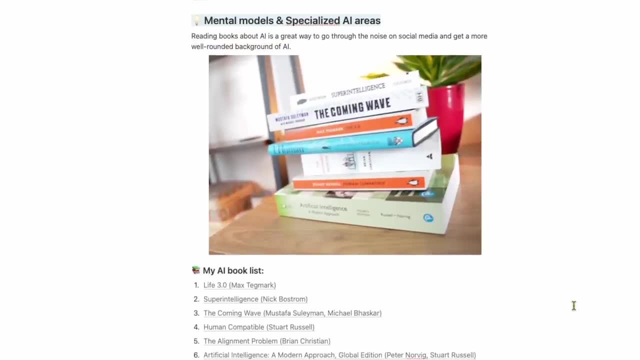 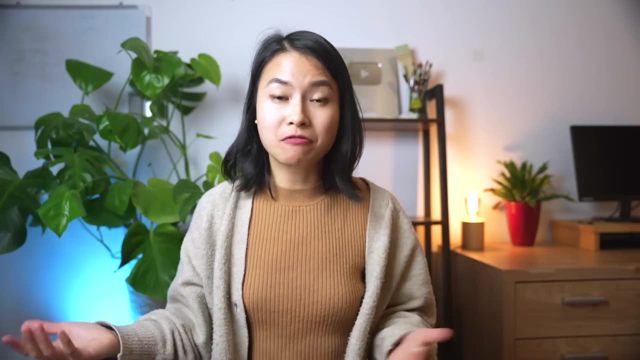 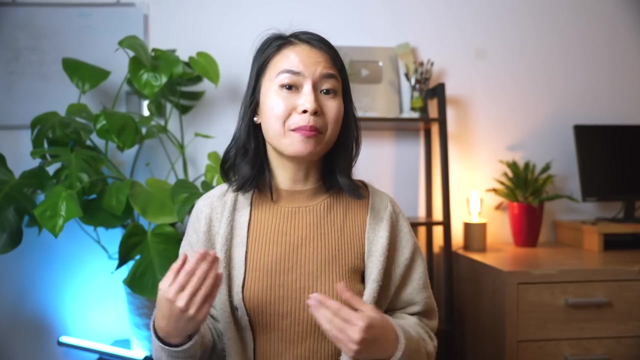 interpret things that you see or hear about AI today. You can also find my AI book list in the roadmap. Personally, I also find it so crazy how much important stuff around AI that is not talked about more widely on the mainstream media. There are many topics around AI that don't make headlines. 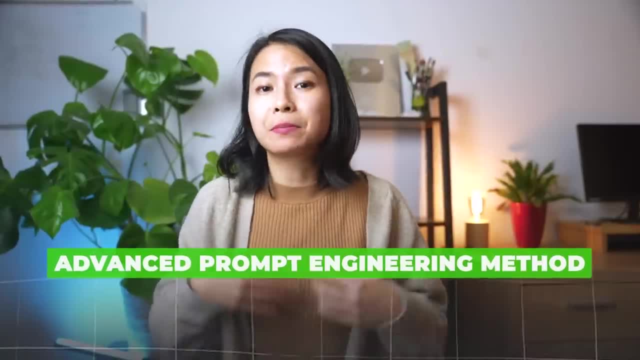 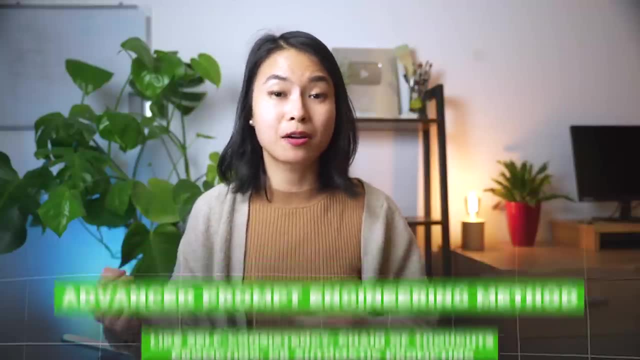 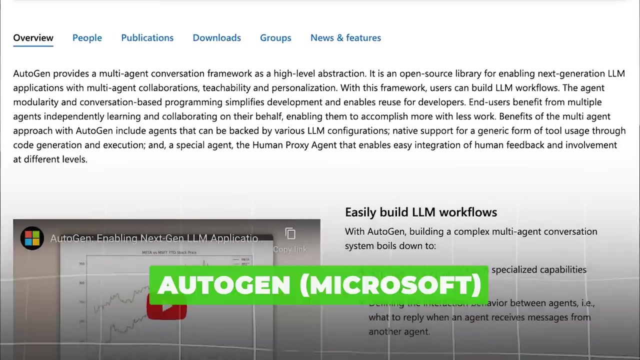 For example, advanced prompt engineering methods to improve the quality of the LLM response, like self-consistency, chain of thoughts prompting or automatic prompting- Autogen- project by Microsoft that allows you to develop LLM applications using multiple agents that can work with each other to solve tasks. Advanced document QA with multi-modal documents that